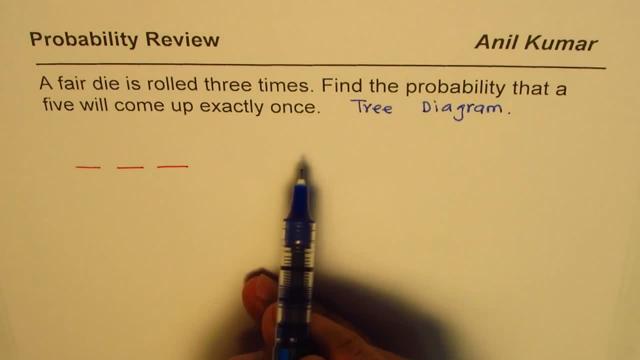 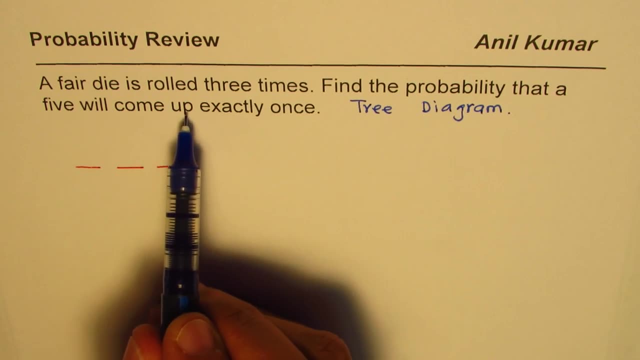 I am adopting counting principles to find the probability that a five will come up exactly once. Find the solution of this particular question. Now. when we say find the probability that five will come up exactly once, that means five will definitely come. It could come in the position first, second or third, right. So we will consider three options. 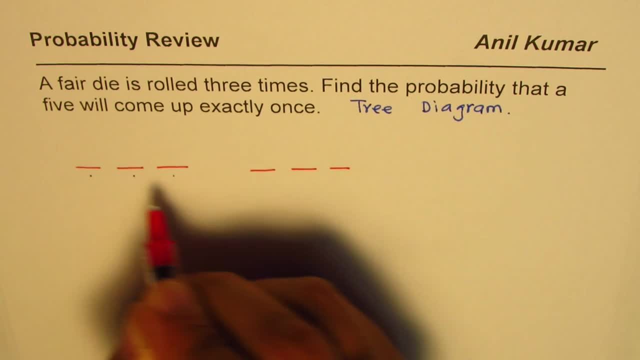 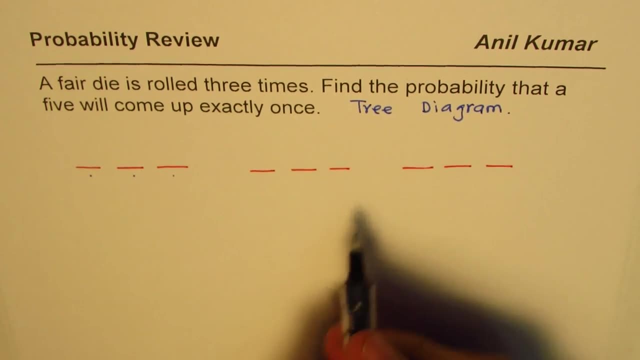 So we have three options. It could come either in the first position or in the second position, or in the third position, right? So that is the probability And these three cases will. we will see what they are and then we will just add them up. 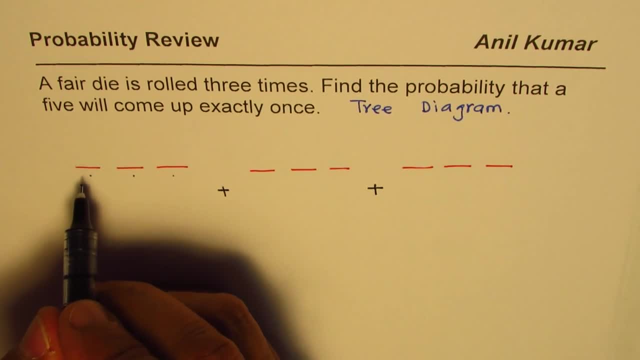 right to get our final probability. Now, if five comes one in the first position, what is the probability of getting five here? It is, we are getting five here, so it is one out of six, right, So it is one out of six. If we get five here, we want five in, exactly. 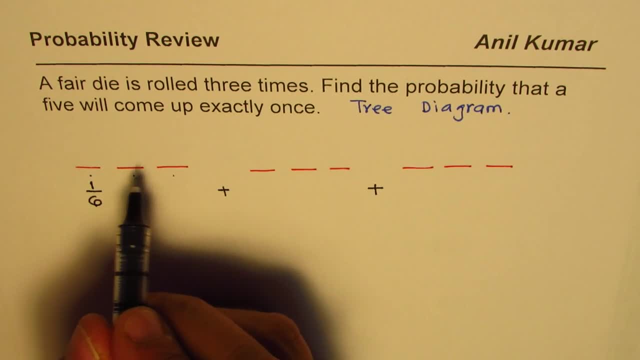 one position. So these two positions are occupied by other numbers, that is, 2,, 3, 4 or 6, 1,, 2,, 3,, 4 or 6.. So other five numbers. So the probability of getting those numbers will be 5 out of 6 or 5 out of 6, right. 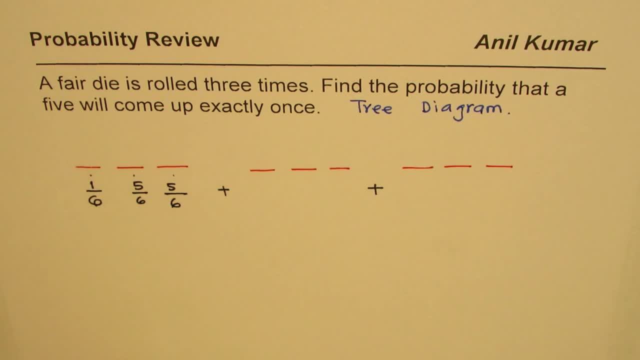 So, from counting principles, probability of getting 5 in the first position- let me write down: 5 in the first position, therefore, is product of these. that is, 1 over 6 times 5 over 6 times 5 over 6.. 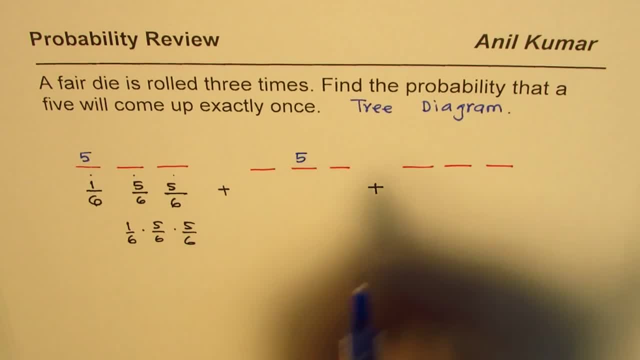 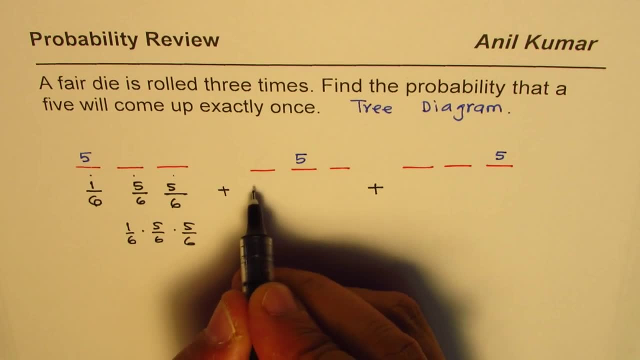 Now, in the second case, 5 could come in the second die and here it could come in the third die, So the probability will be here. we could get any other number, So it will be 5 over 6 times. there is only 1 out of 6 to get us 5.. 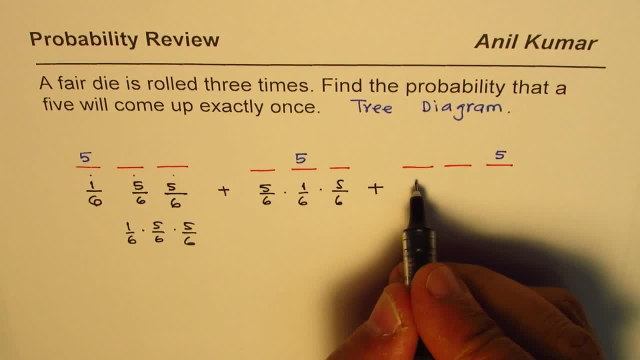 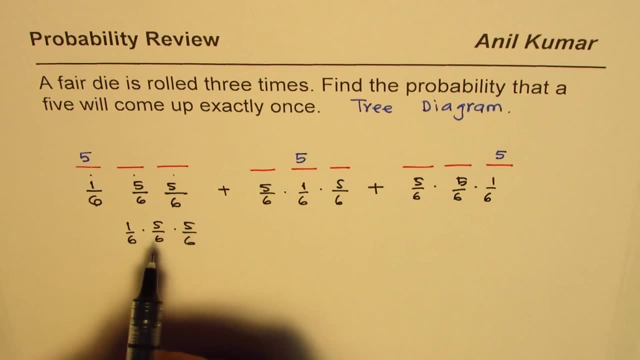 And 5 numbers could fall Similarly. here it will be 5 over 6 times 5 over 6 times 1 over 6, right. So it is kind of same thing: 3 times right times times 3..